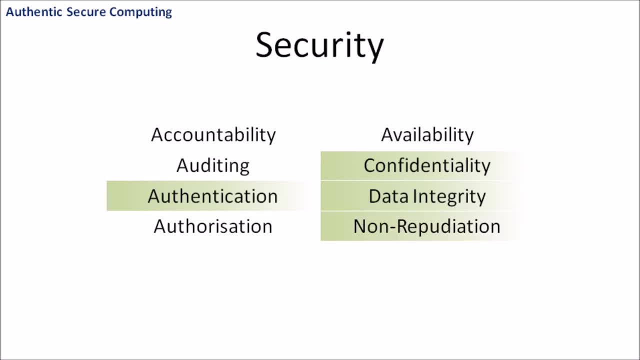 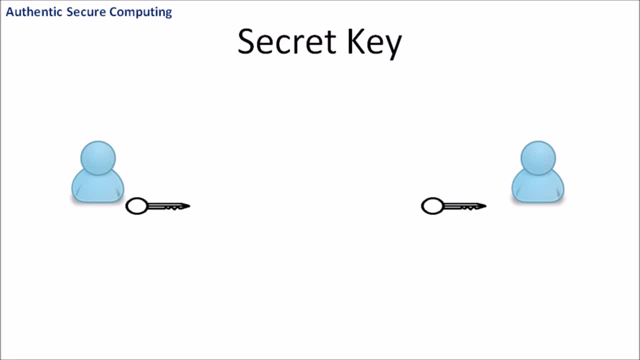 Non-repudiation means that the sender cannot deny sending the message. There are four classes of cryptographic algorithms. The first is secret key cryptography, which is also known as symmetric cryptography, because both communicating parties must have the exact same keys to communicate. The communicating parties use a pre-shared 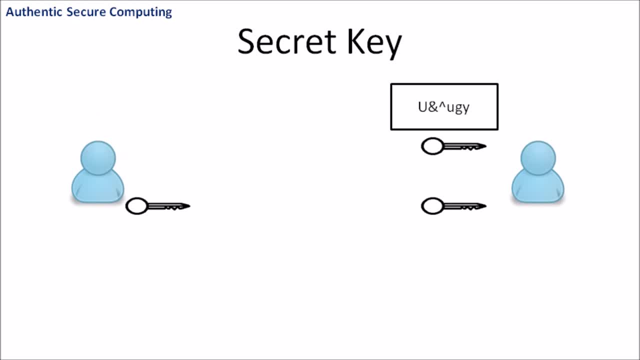 key to encrypt and decrypt the message. The second is public key cryptography, in which the public key of the communicating parties are publicly known Like secret key cryptography. there are many different algorithms for this type of cryptography. For the purposes of this video, the RSA algorithm is used. 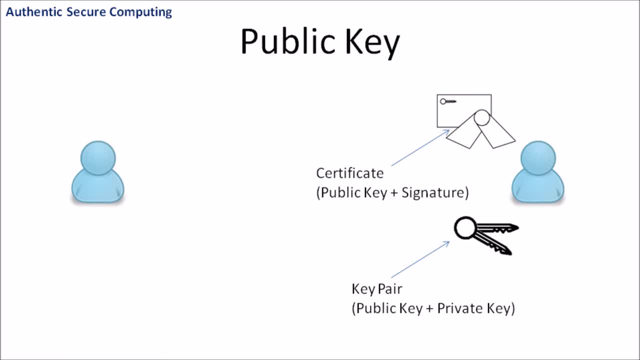 The feature in public key cryptography is the message can only be decrypted by the private key that is only known to the party that generated the public private key pair. Additionally, public key cryptography can be used to sign and verify messages. Messages that are signed using the private key can only be verified by the public. 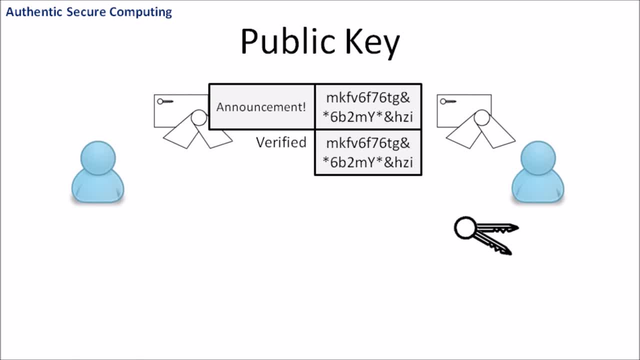 key from that particular private key. Therefore, the recipient of the message has full confidence that the message was created by the communicating party and not by an adversary. A trusted party that signs and holds the certificates of the communicating parties is then known as the. 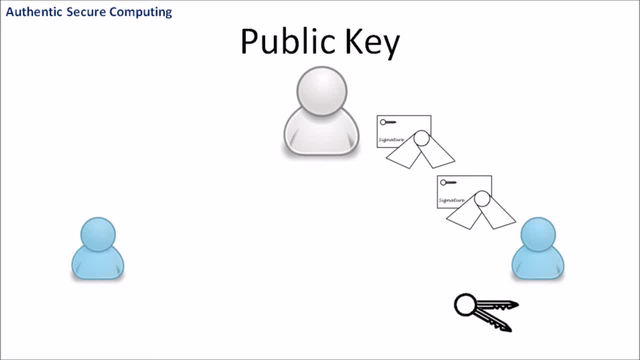 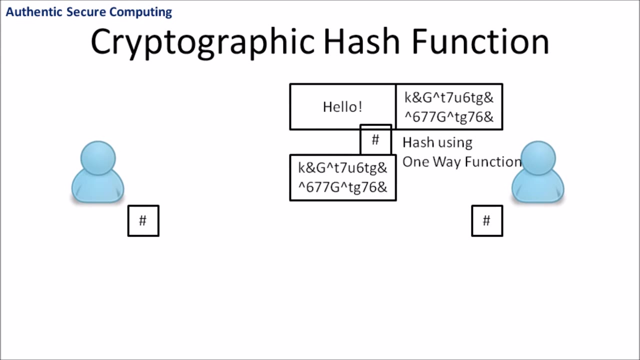 certificates authority. The certificates authorities are trusted entities that signs all the certificate signing requests. The certificates are then trusted until they expire or are revoked. The third class is known as cryptographic hash functions, which is a one-way hash function that generates a bit string. deterministically, Hash functions are typically. 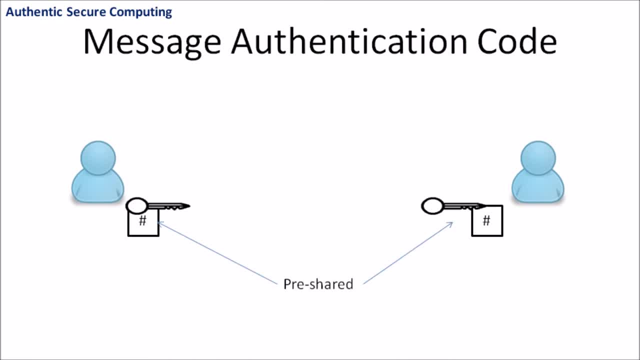 used to verify the data integrity. Finally, there's message authentication code, which is very much like the cryptography. However, it incorporates the use of a pre-shared secret key so that the sender and recipient can authenticate the cryptographic hash value upon receipt, Since the secret key has an 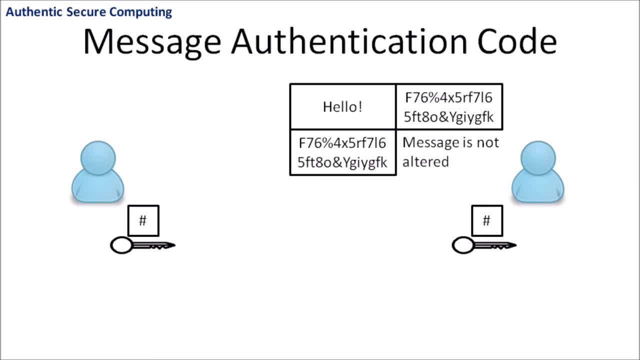 effect on the message authentication code that is generated. only the parties with the secret key are able to check if the message authentication code that was received by another party is a match Secret key. cryptography is rarely used alone for communications because of the key management problems.